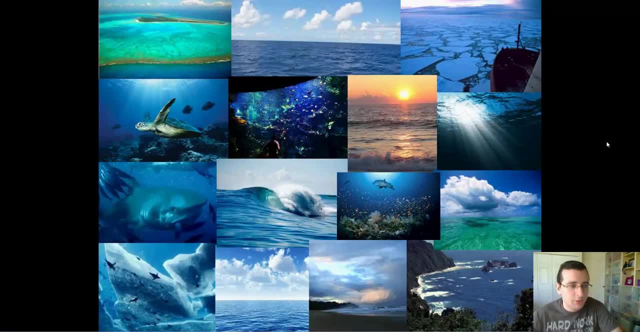 So it's about oceanography, and you see here some beautiful pictures of what, in my opinion, is the most beautiful part of our planet, And it's what makes our planet so unique too, the fact that it's covered with oceans. Now, these are the oceans of the world. There are five major oceans in the world. 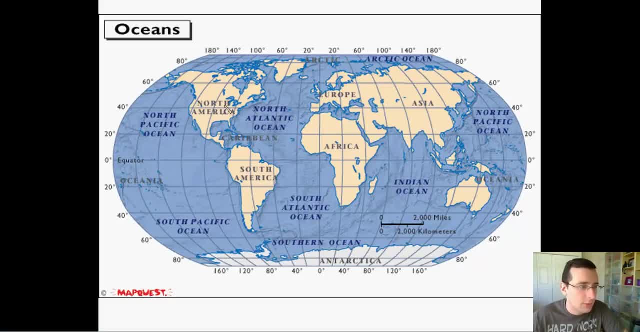 We have the Atlantic Ocean, which is in between the two major continental blocks, between the Americas and the African-European blocks. So there you go, you have the Atlantic Ocean right here. Then you have the Indian Ocean, In between the Oceania, Asia and Africa. 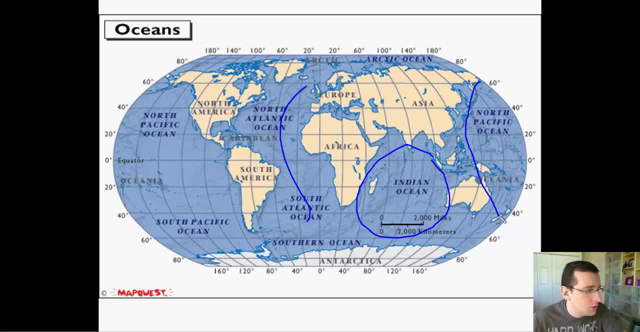 And then you have the large Pacific Ocean, which is in between Asia and Oceania and the Americas over here, And that's definitely the largest ocean in the world. Now in the top you have a small ocean called the Arctic Ocean. 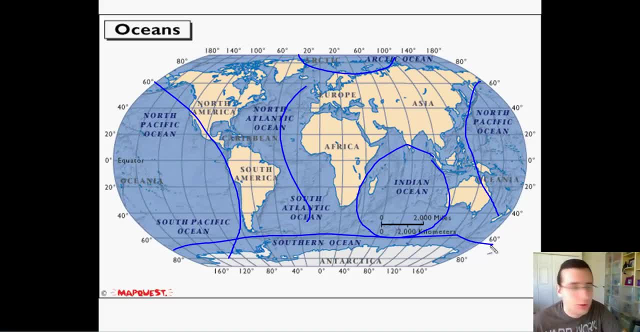 And in the bottom you have the Southern Ocean, also called Antarctic Ocean. So those are the oceans of the world. make sure you know it. Now I'd also like to point out that there's also something called seas. Have you ever heard about the seven seas? I'm going to sail the seven seas. 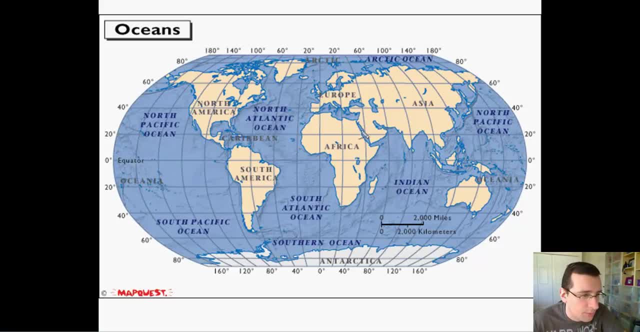 Well, there's way more than seven seas, And I'm going to show you some examples of seas. Here you go: you have the Red Sea right. You have the Arabian Sea. You have another sea right there, You have the Asiatic Sea right there. 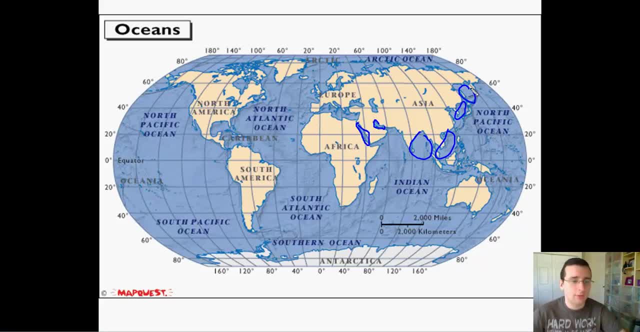 Sea of Japan right there. You have the Russian Sea right there. You have the North Sea right here. All right, you have the sorry, the North Sea is right there, but you have another one there. You have another sea right there, another one right here: Mediterranean Sea right here. 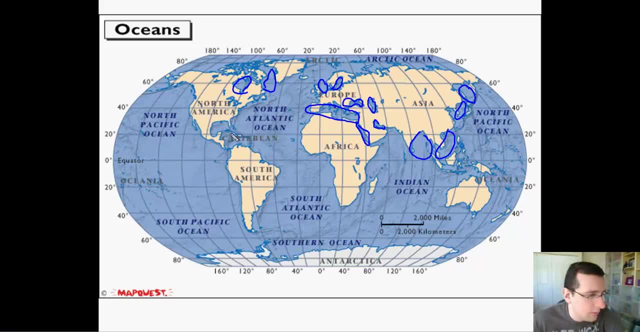 another one there, another one here. Caribbean Sea, right there, right? So what do you see in common in these seas of the world? Seas are chunks of the ocean which are isolated or mostly surrounded by oceans. They're surrounded by land. Look at the Mediterranean Sea as a perfect example. 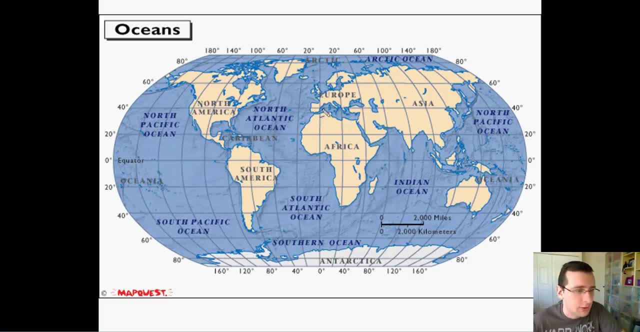 It's almost completely surrounded by land, which means they have their own currents, their own evaporation rates, their own animal life, their own characteristics. So they're like mini oceans within the world and they actually differ a lot from the oceans they belong to. 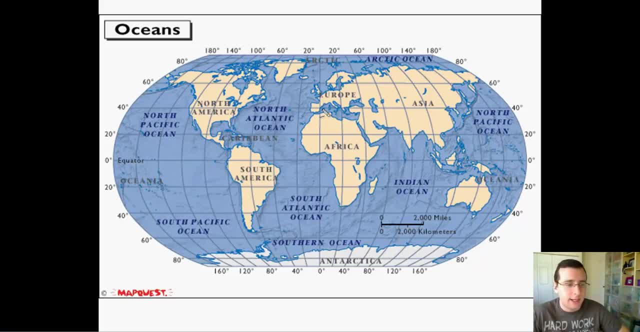 So, for example, the Mediterranean is attached to the Atlantic Ocean, but it's very different from the Atlantic. The Sea of Japan is attached to the Pacific Ocean, but it has very peculiar features. It is not actually under the influence of Pacific currents. and so you're going to. 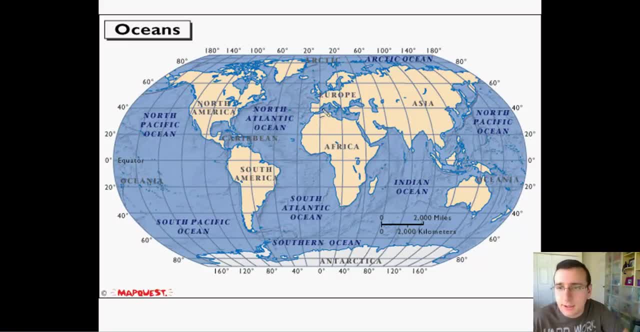 have different setups. The same thing with the Caribbean Sea. It's usually hotter than the Atlantic as a whole and it's not really part of the Atlantic Ocean current belt. So, as you see, these seas are chunks of the ocean. So that is what we talk about when we talk about seas. 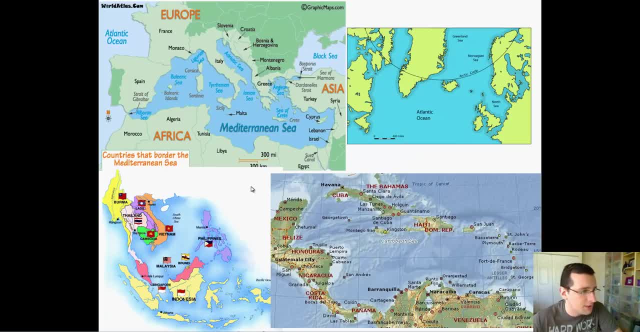 So here you see another representation of this. The Mediterranean Sea is surrounded by Africa, Asia and Europe and it's right in between those continents and it's almost completely surrounded by ocean. Even the Mediterranean is actually split into other seas. because you can see that you have 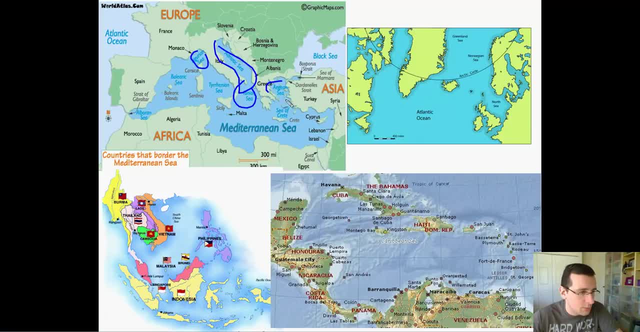 an area there, an area here, another one there. Each one of those areas, they're peculiar currents. So people actually have historically split the Mediterranean Sea into smaller seas. You also see another sea right there, the Black Sea, Which is also. it has its own current, so it's connected to the Mediterranean by the 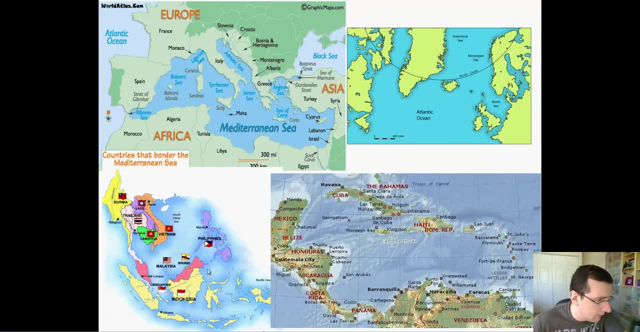 Bosphorus Strait. Here you see the South China Sea, which is in between the Indonesia and the southern peninsula of the Asiatic countries, And China would be right north of that. And then look here at the Caribbean Sea. You see how it's surrounded almost completely by islands and land. 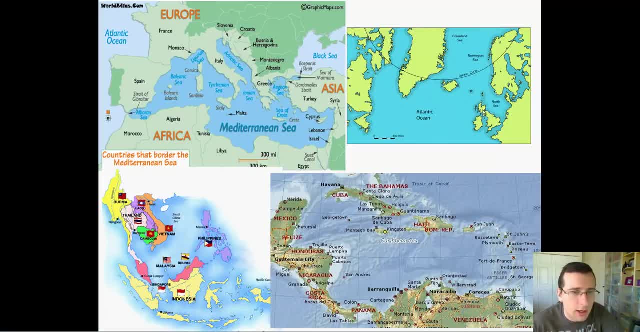 It's surrounded by the Pacific Ocean On the Americas And- look there, the North Sea right there. You also have the Scandinavian Sea on the right side and you have the Greenland Sea and the Norwegian Sea, and then you have the Canadian Sea up there as well. 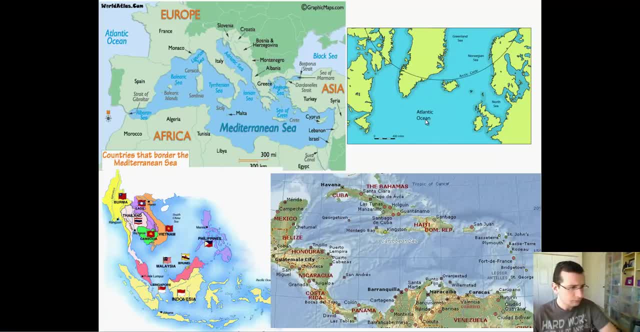 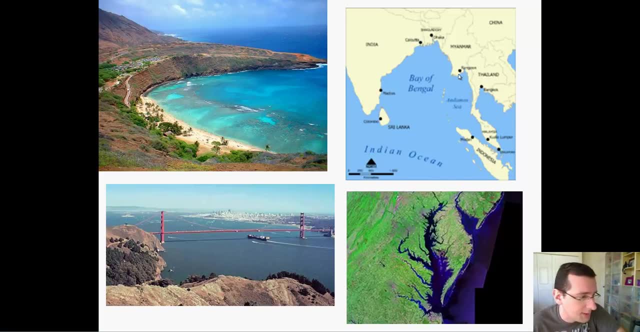 So you see, seas are isolated pieces of the ocean. all right. Now you also have bays. Now bays are not quite seas, although a lot of seas can form within bays. but bays are either small or large, And bays are large incursions of water into the land. 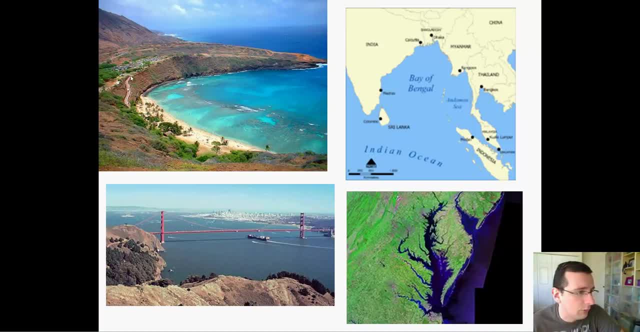 So, for example, you have in the screen here a small bay, where you have- you actually have a peninsula stretching from the earth into the thing, which creates a bay surrounding that. You see that, And then here you have the San Francisco Bay. 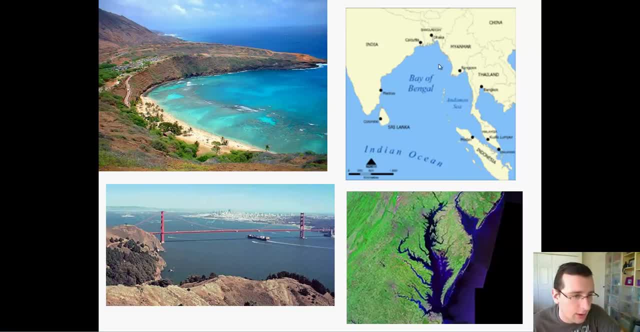 You have the Bay of Bengal in China, in India, which houses the Andonian Sea, And then you have the Chesapeake Bay right here in the US and another bay right there as well. So you see that bays are incursions of ocean into the land. 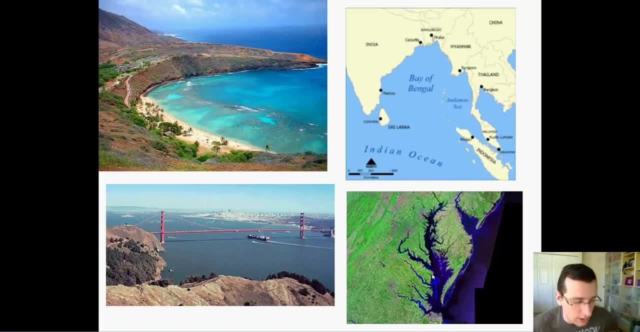 And if they're large enough, they can actually form a separate sea, And that's pretty much how we what we have. okay, So that's a bay. Now, if a bay is really large, we call it a gulf, like the Gulf of Mexico or the Gulf. 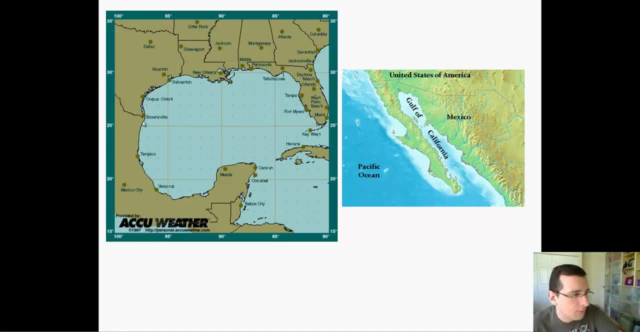 of California which actually forms. it's an extremely large bay, almost to the point that you could call this its own sea. And yes, you could. You could theoretically call this the Mexican Sea, but although nobody does, And then you see, the Gulf of California is also a large, large, large, large bay. 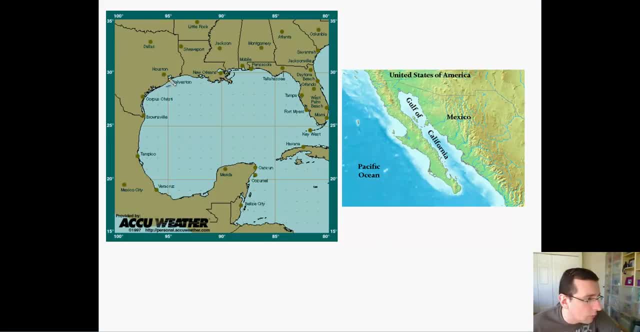 Now, meanwhile, look here at the Gulf of Mexico. You see smaller little bays. Look, there's one right there, there's one right here, there's one right there, You know. so, there's one right here. These are bays. 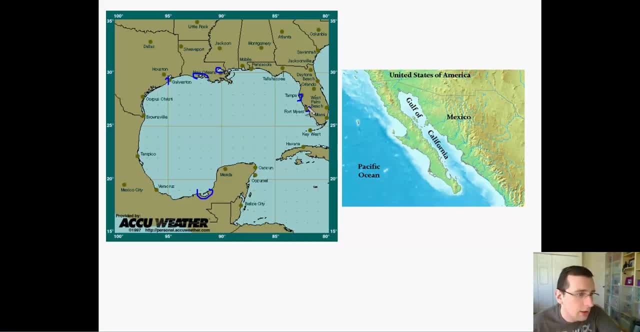 Look at Florida, It's all. you see Tampa Bay, you know Fort Myers Bay, You know there's a bay right there as well. So their bays are usually small, small But But you can have large, large bays in a large scale. 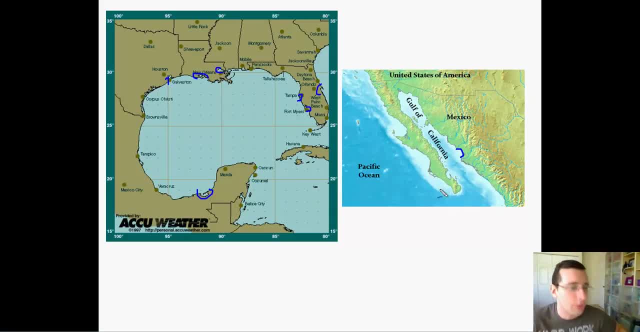 Look at the Gulf of California. You can have a smaller sub-bay right there as well. So bays are incursions of water into the land and which can form their own seas, and if they're really big, we call them gulfs okay. 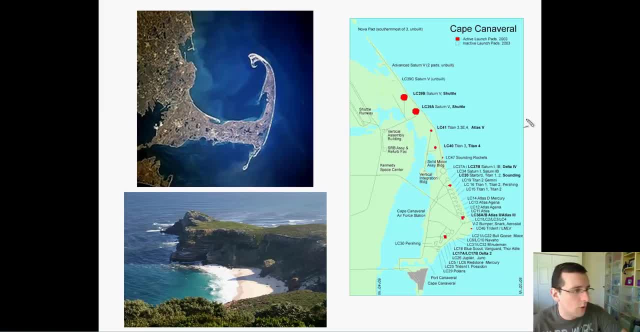 Now the same thing. we have the word peninsula. Now a peninsula actually helps form a bay. So, for example, you see, over here I see a bay, but it's actually formed because of a large peninsula, which is a stretch of land that's going into the sea. 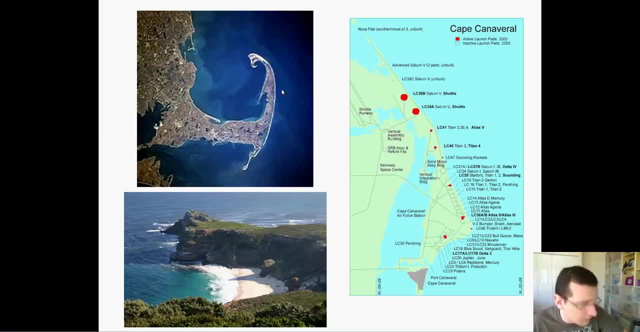 Just like a bay is a incursion of water into the land, uh, peninsula is an incursion of land into the water, and it's usually connected to the land by something called isthmus. So you see, here it's a narrow stretch of land that actually connects the peninsula. 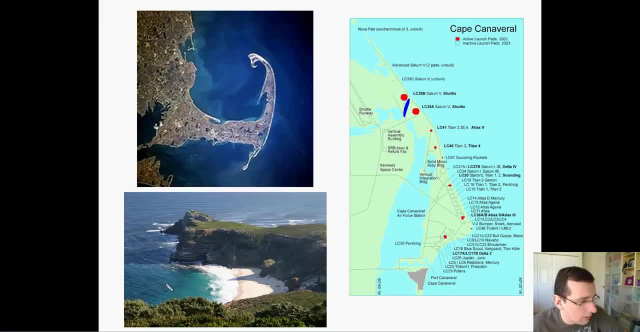 to the continent, And so that's why we call it a canista. Now see here again: a narrow stretch of land that connects the peninsula to the to the continent. A narrow stretch of land that connects the peninsula to the continent. 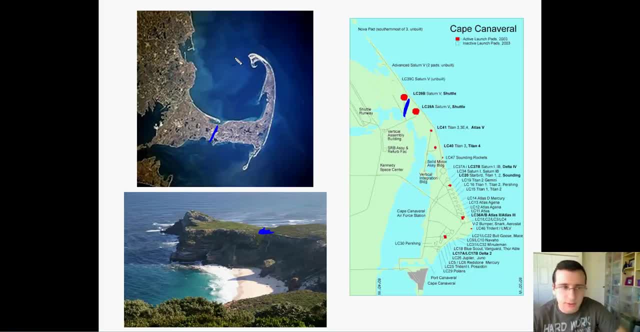 Excuse me, Kind of like what it is. And another word for peninsulas is cape. So you see, Cape of Good Hope, Cape Canaveral, Those are good examples of it, And actually this one in the left, the right corner is actually the Cape of Good Hope. 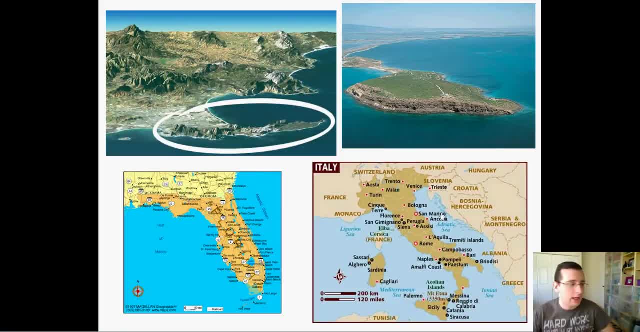 All right. So then we have- here are more examples of peninsulas. all right, You have a large, large stretch of land and a narrow bridge connecting that right. Here's another one right there, an isthmus that's connecting that peninsula to the land. 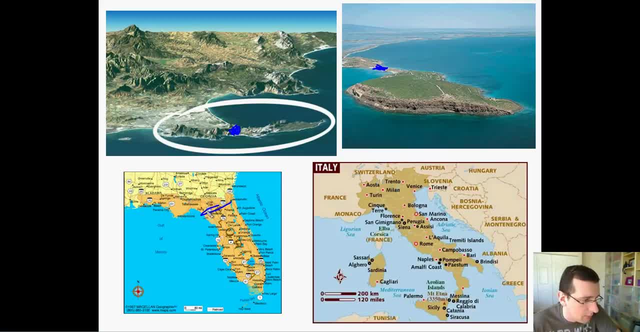 Florida in itself is also a peninsula because it has a small narrow bend of it connecting to a large continent. Look at the same thing for Italy: It's a peninsula, So you see how they can actually form large bays and oceans and things like that. 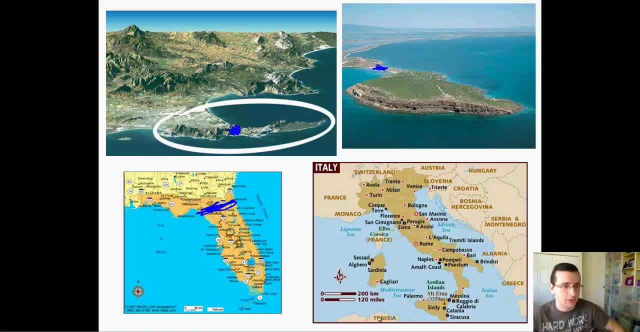 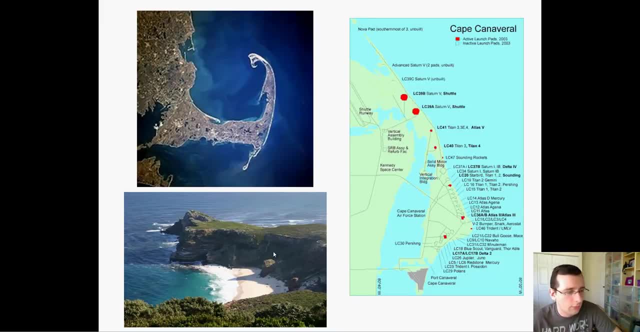 So that's the goal. Now, remember that bays are technically small, It's just like capes are small: peninsulas. So you see here, on the previous thing, Cape Canaveral and Cape of Good Hope as good examples of peninsulas. 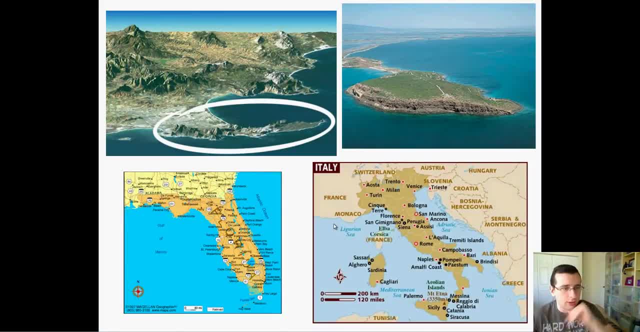 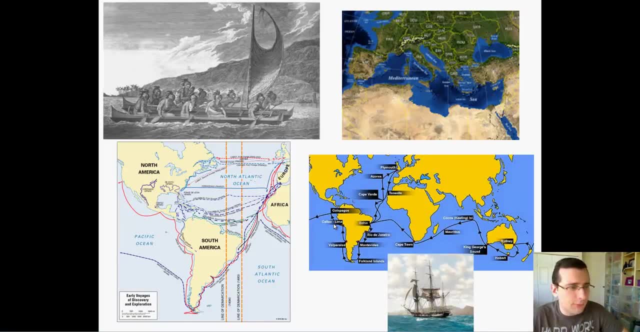 Now let's talk about capes, which are small peninsulas- all right, large peninsulas you see here in this screen. Now let's talk about the history of oceanography. all right, The first people to try to seafare were the Polynesians. 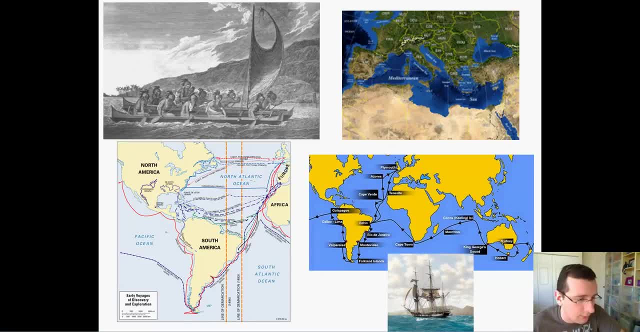 The Polynesians were Indian- well, we call them the native Indians- but basically they stretched from the Americas into Asia, into the islands of the Pacific. So the Polynesian people were the first large seafarers. Even before that, historically, you have people trying to conquer the sea in the Mediterranean. 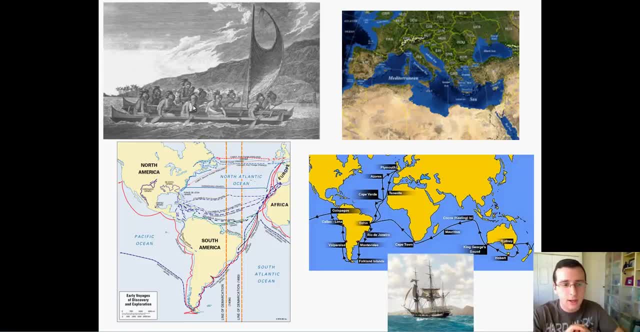 You have Greek battles and Persian battles in the Mediterranean. You have Egyptians trying to make that Naval navies on the Nile. So navies are not as ancient things, but the first ones to cross continents were definitely the Polynesian people. 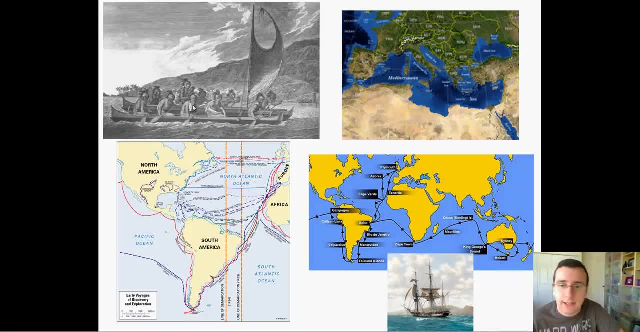 And then you have the Vikings with Leif Erikson and other things like that, which actually went from Europe to Greenland and then finally to the Americas in Newfoundland. all right, So these are just examples, But Mediterranean Sea is another example of area of the world which was there were great sea exploration even before the Common Era. 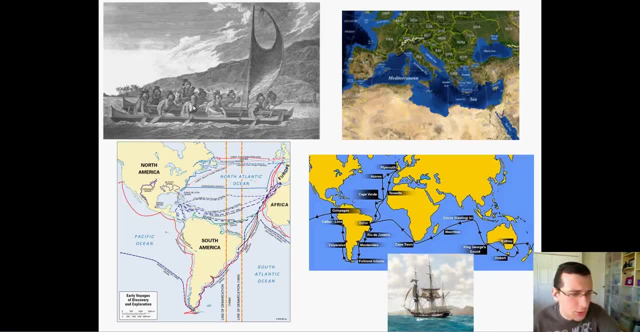 So even before Christ used to have the seafarers going there. But the Polynesians were the first ones to really become seafarers that conquered a lot of islands on the Pacific. In fact, by the time the Europeans found those islands in the 1500s and 1600s, Polynesian people had already been living there for hundreds of years. 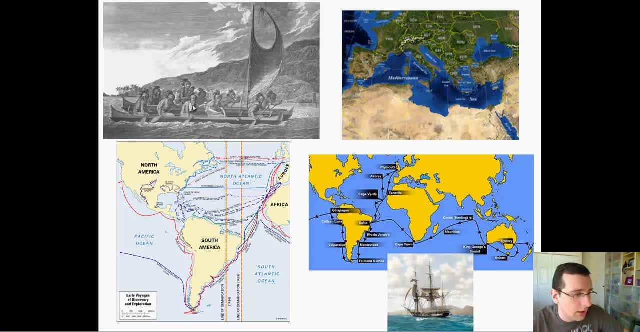 Now the Age of Discovery started with the exploration of the West and the need to try to reach India through the actual East. So they actually headed India was on the East and they wanted to get there. but they actually- people like Christopher Columbus- actually believed that heading West you could get to East. 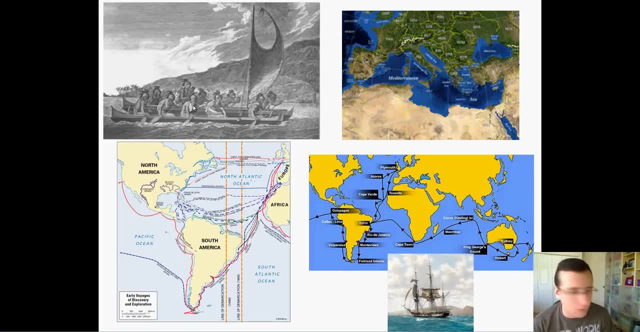 And it was faster because the Earth was rounded, And so began the large exploration of the world. And you have all those famous explorers like Ponce de Leon, Vasco da Gama, Columbus, Leif, Erikson, Americo Vespucci, Cabot, Drake, Cartier, Chaplain, Cortes, Hudson, Magellan, Coronado, Pedro Alvarez, Cabral, Marco Polo. 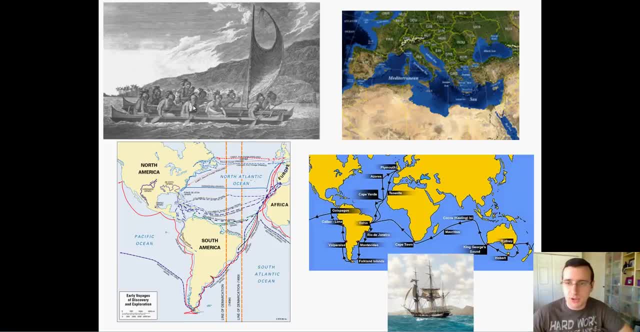 a bunch of explorers that have taken to the seas and advanced the exploration of the seas, navigation, understanding of currents, Understanding of how the wind creates waves, And all of this led to the more and more understanding of the oceans. So, as people were trying to conquer the Mediterranean Sea, Polynesian people trying to travel around the world, 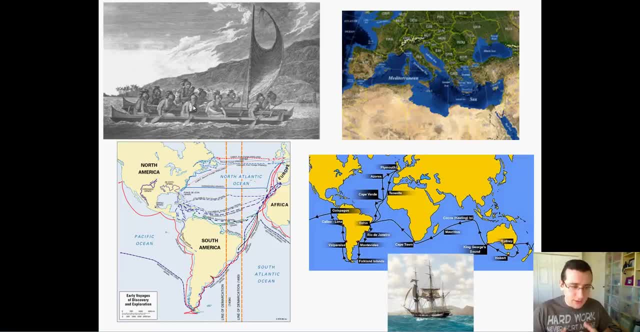 and the great explorers of the Age of Discovery. you have these more understanding of the oceans because of it, For example, the Charles Darwin expedition on the HMS Beagle, which you see on the right hand side here of the screen- they actually went around the entire world and they had to understand something. 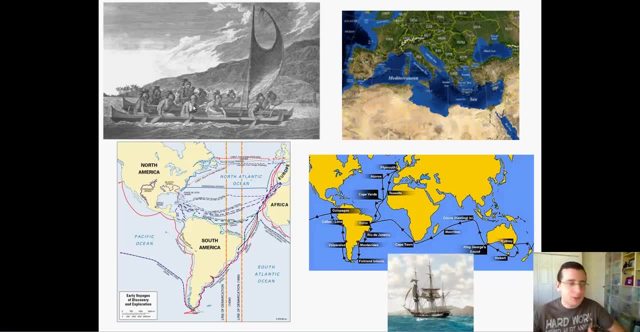 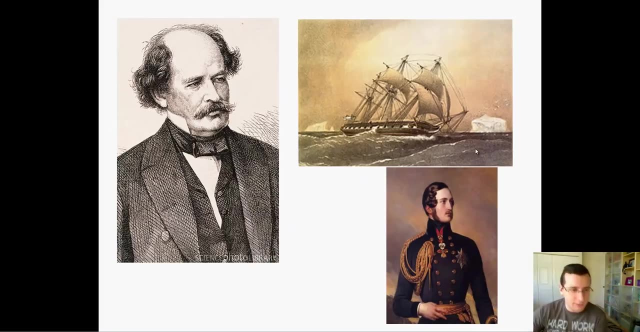 They had to understand something about the ocean and how it works in order to do that. So with the Age of Discovery and more and more sea exploration through ships powered by wind, the understanding of our oceanography actually increased. But it wasn't until the Challenger expedition, the HMS Challenger. this ship here you see, on the top right side. 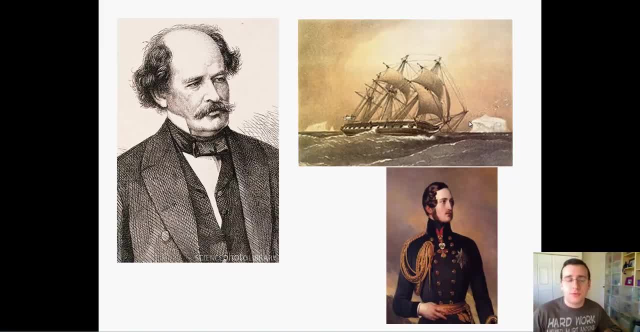 that, for the first time, a group of scientists went out to the oceans with a dedicated mission of understanding the oceans. Over 200 scientists- Over 200 scientists- joined a crew of the HMS Challenger and this was the first ever oceanography expedition which was launched with the purpose of understanding currents, studying the depth of the oceans. 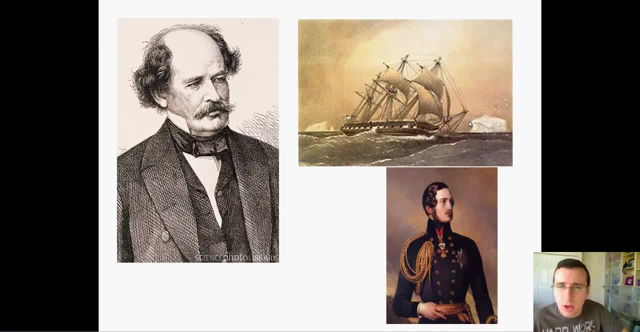 studying how waves are formed, what causes tides, all those kinds of things which we're going to actually be learning about now. And two of the most prominent early developers, which are also involved in the Challenger expedition, are Prince Albert and Matthew Morey. 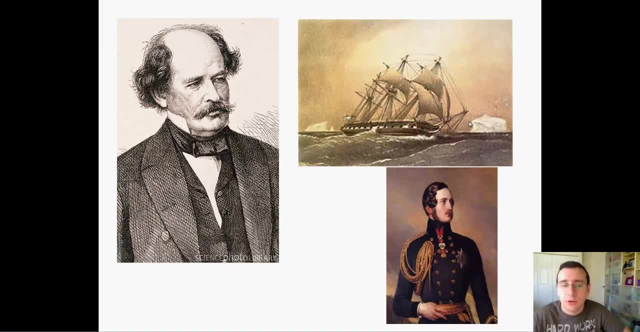 which were? they were mappers of the currents of the oceans and they were trying to understand how these things worked in order to better understand- And we were talking about late 1800s here, Even way past the Age of Discovery, way after Charles Darwin and other great explorers explored the oceans- 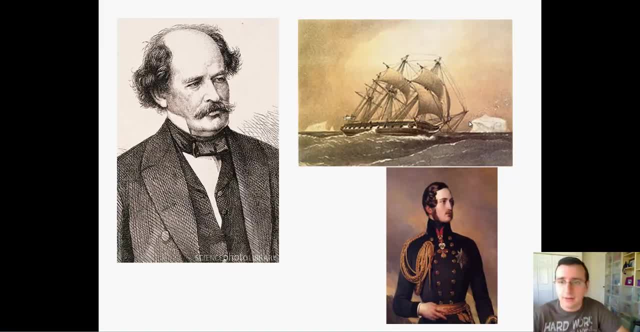 this is when they actually, for the first time, sent a dedicated message And that most people considered the birth of oceanography as an actual field of science. Because the discoverers- yes, they learned a lot about the oceans. Yes, the commerce of the West India, trading and all these things. 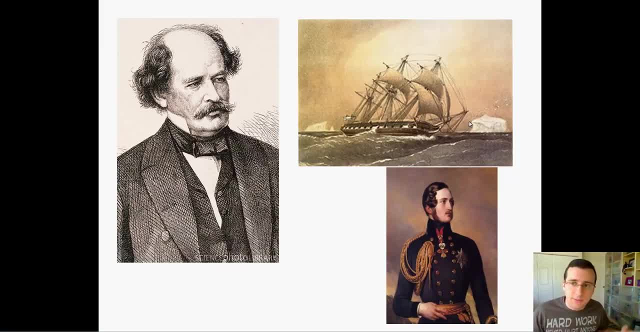 All the they advanced. you know the seafaring Pirates of the Caribbean. you saw the movies. All of that advanced the understanding of the oceans. But it wasn't until the Challenger expedition and Prince Albert and Matthew Morey that oceanography was born. 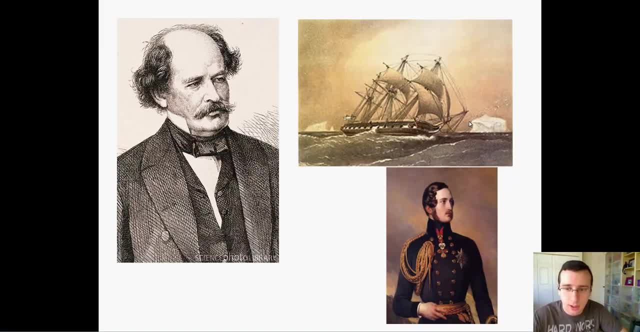 Which is why Matthew Morey is considered the father of oceanography Now after him, for the last hundreds of years and since, actually, the beginning of ocean seafaring, since the Mediterranean. you remember I told you about great battles between the Greeks and the Persians.